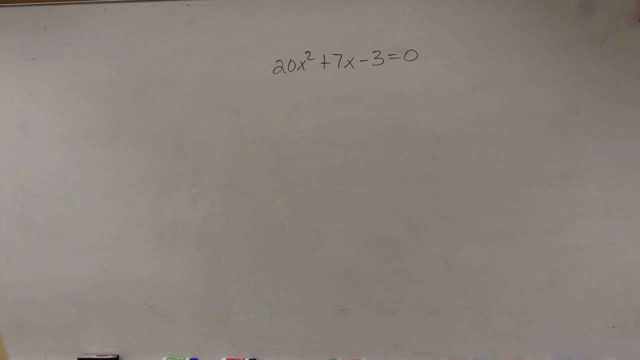 Alright. so for this problem, I have 20x squared plus 7x minus 3, and the main important thing that I'm going to want to do is make sure that it's in quadratic form, or it's a quadratic equation, which of course it is. We can write this as: ax squared plus bx plus c equals 0.. 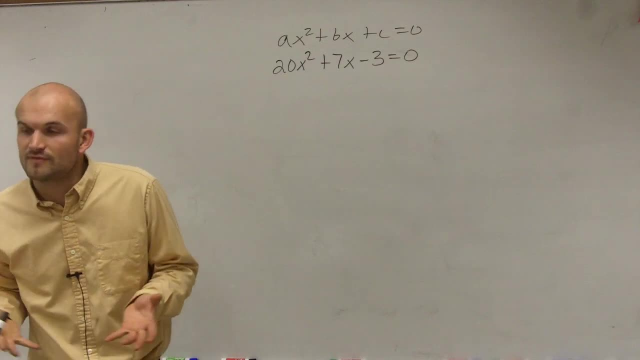 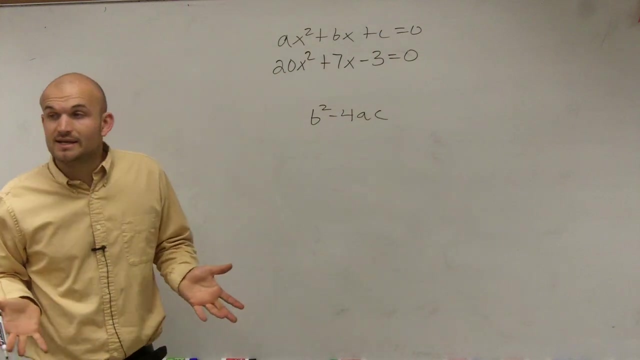 So once I have it in that form, the first thing they want us to do, Wendy, is to be able to find the discriminant. Remember, the discriminant is written as b squared minus 4 times a times c. So to do that, I need to make sure that I know what my a, b and c. 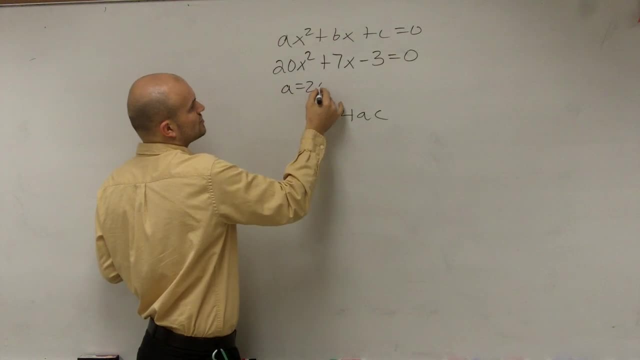 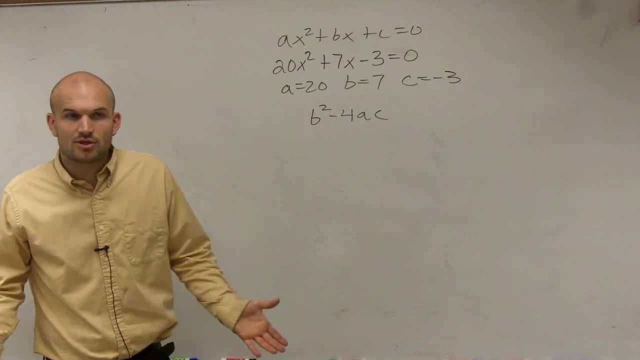 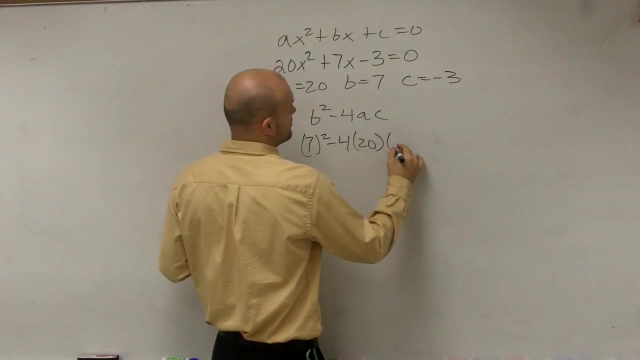 are Well, by following my quadratic equation, I can say: a equals 20,, b equals 7, and c equals negative 3.. Therefore, now let's go ahead and just plug in the values. So we have 7 squared minus 4 times 20, times c, which is negative 3.. Alright, so now what I can do. 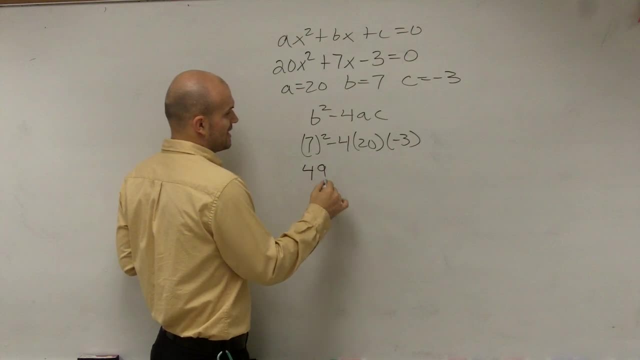 is just go ahead and simplify, Ricardo. So when I do that, I have 7 squared minus 4 times c, So I have 49 minus 4 times negative. 20 is going to be a well hold on, Let's just. 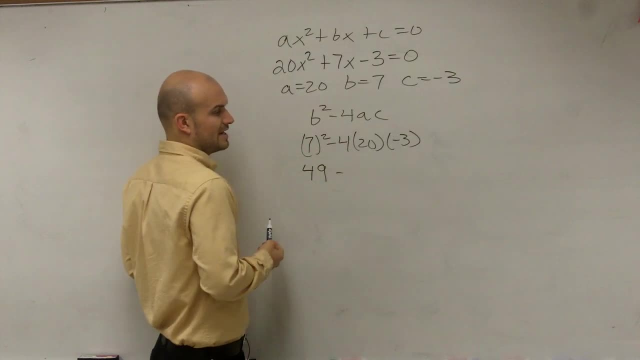 do it this way. Let's do 20 times negative. 3 is going to be 20 times negative. 3 is going to be a negative 60.. Negative 60 times a negative 4 is a positive 240.. Do what? Yeah, That's. 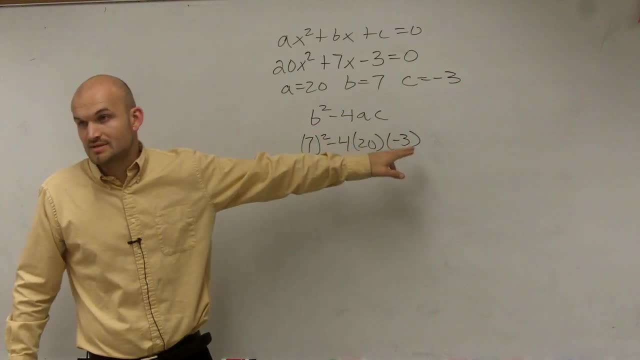 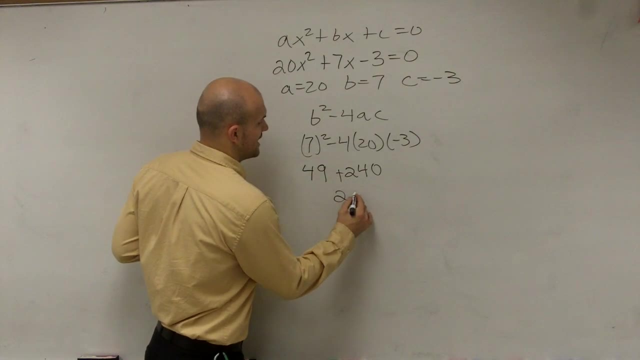 a negative 4.. Negative 4 times 20 is negative 80.. Negative 80 times 4 is a positive 240.. Negative 80 times negative 3 is a positive 240.. So I'm really actually adding 24 plus 240, which would give me 289.. So now what I need to do is determine: is that a square? 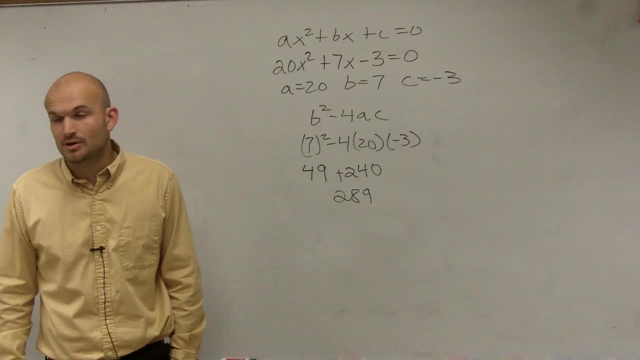 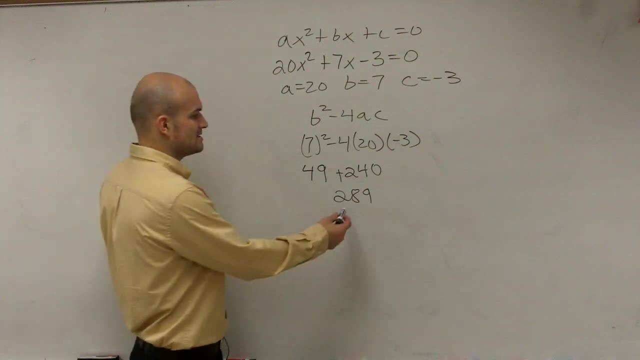 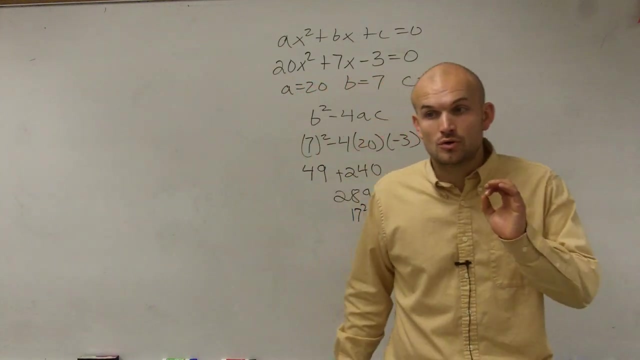 number within itself. Is that a number multiplied by another number? Yes, And what is it? So you can look at this and you can rewrite this as: yes, 17 squared. So, since it is a square number, 17 squared, we know that we're going to have two real radicals, So we're 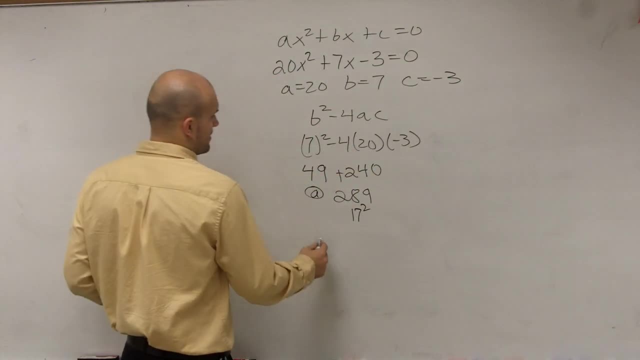 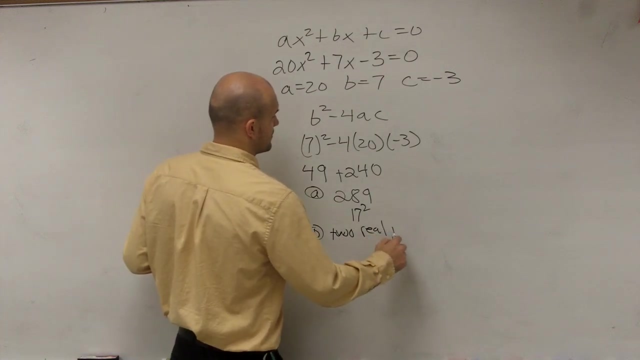 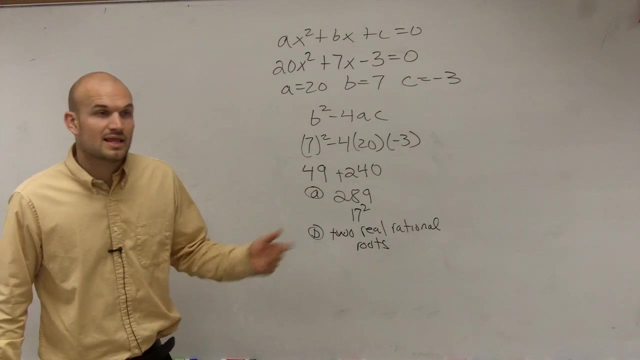 going to have two rational roots. So that was A, Then for B, you had to describe it. So, yes, we have two real rational roots. All right, Then the last thing C said to actually evaluate for the answer. So what we're going to do is we're going to apply this to the 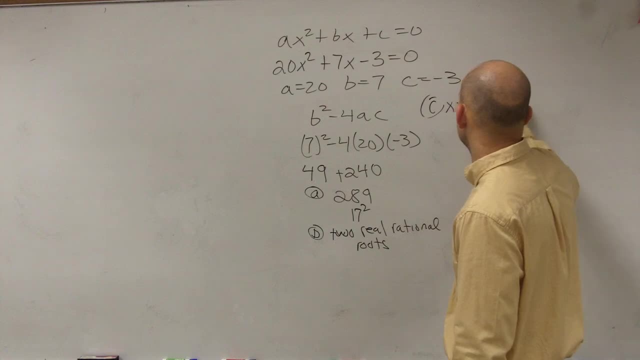 quadratic formula. So the only thing we need to add now is opposite of B plus or minus the square root of your derivative. So we're going to add this to the quadratic formula. So it's going to be the discriminant, which we know is 289, which I'll just write it back. 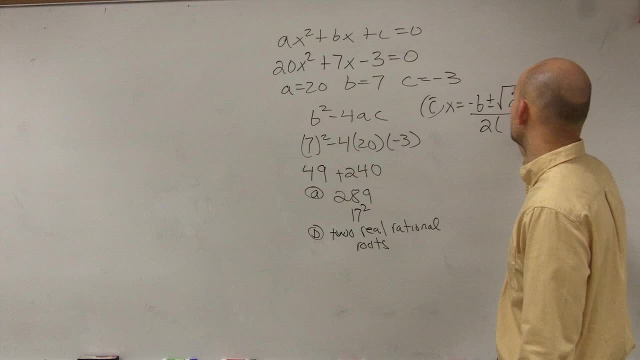 in there, though again divided by two times A, which is 20.. So let's go and plug in our- oh, I guess I could plug in my B too. My B is opposite of B, which is 7.. So therefore, 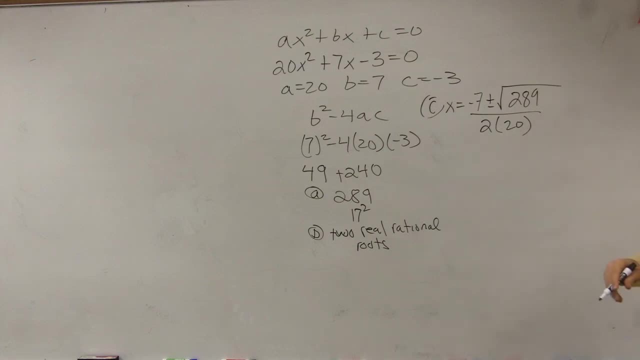 I have, opposite of 7, plus or minus the square root of 289, divided by 2 times 20.. So let's simplify this again: X equals negative 7, plus or minus 17, divided by 40.. All right, 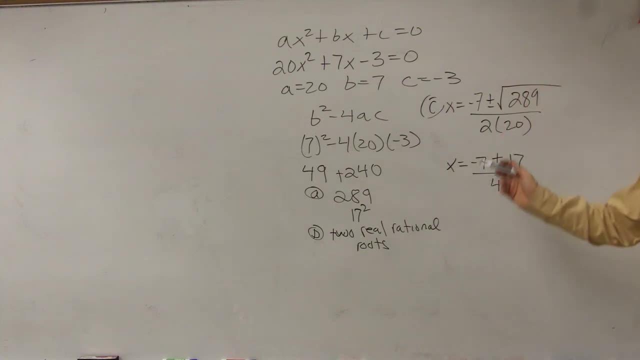 So now, ladies and gentlemen, you can do this either separately or you can do this together. I'm going to add the numerators first and then divide. So negative 7 plus 17 is going to be 10.. So I have one answer: is x equals 10 over 40,, which equals 1. fourth, 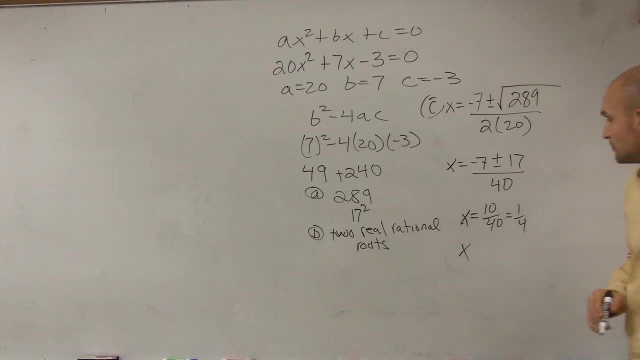 And then negative 7 minus negative 17 is negative 24.. So x equals a negative 24 over 40,, which then you can go ahead and divide by the largest number, which is 4 and 4,, which would be 6 over 10.. 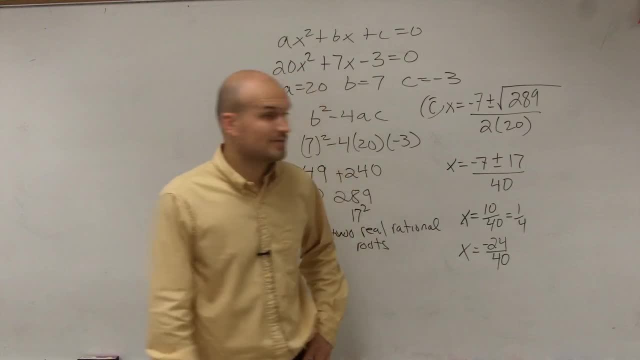 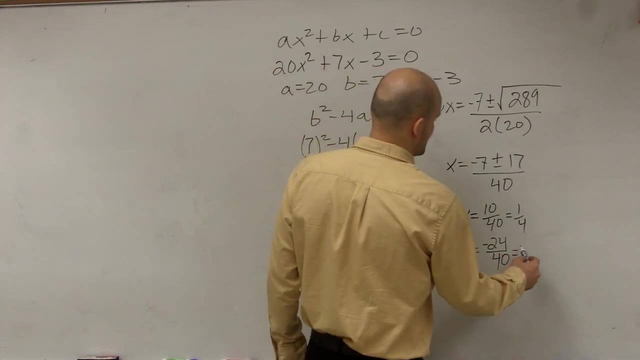 There's what? Well, the largest number that goes into both of them would be 8, right, Because 8 goes into there and there. So, therefore, I divide 8 on the top and the bottom and I get a negative 3 fifths. 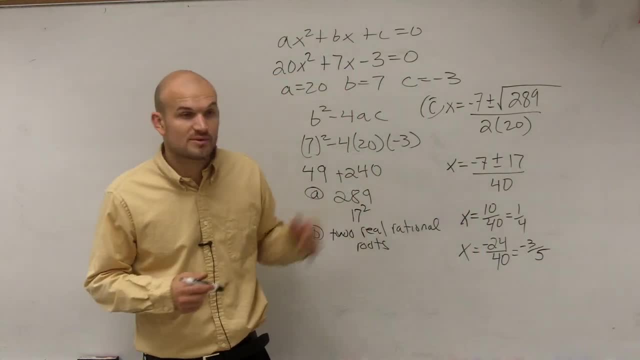 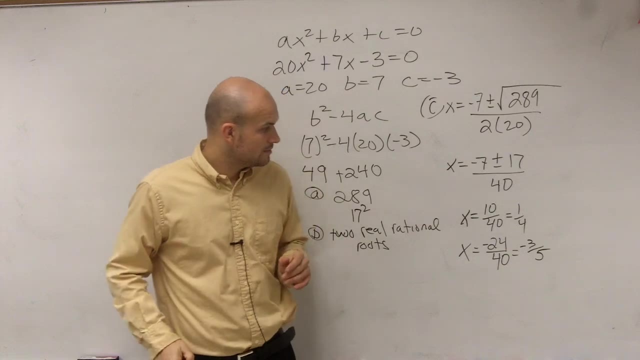 So those are going to be my two solutions to the equation, which also would be my x-intercepts, my roots, my zeros. Yes, Can you not use it? I mean like this, No, I want you to just simplify it to its answer. 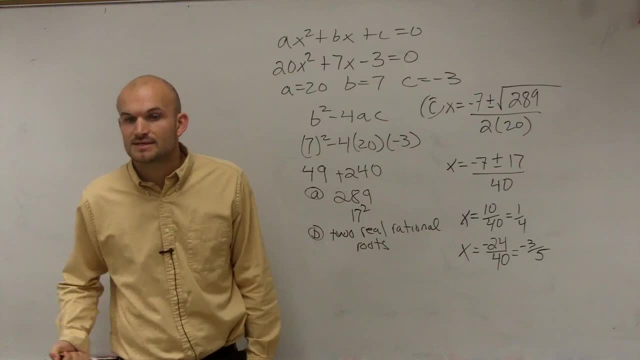 Huh, Yes, it will not be simplified. Yes, So make sure you simplify it.